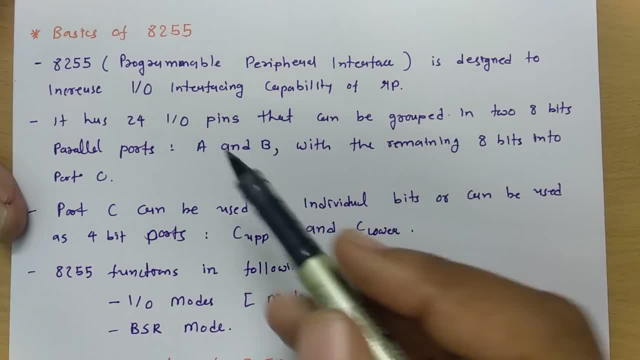 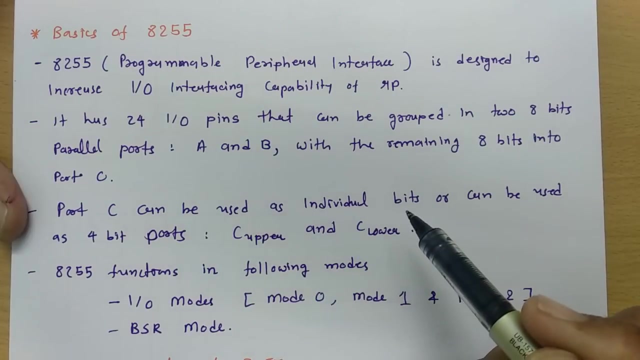 input output interfacing capability of microprocessor. It has 24 input output pins that can be grouped into two 8 bits parallel ports, like port A and port B, and the remaining 8 bits that is placed there with port C. ¿Ports C can be used as individual bit and 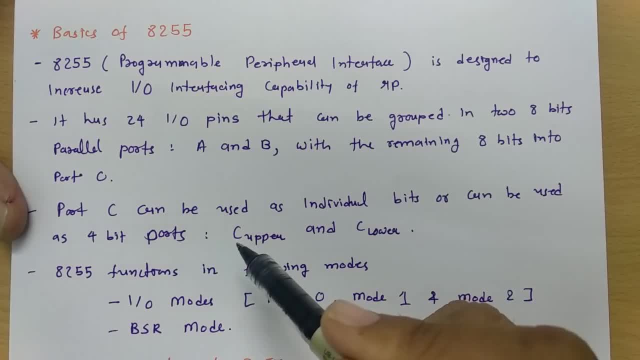 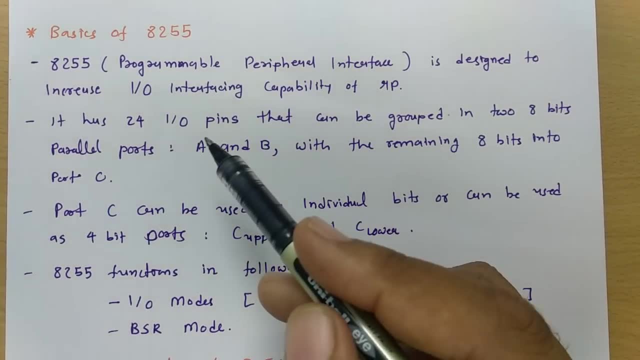 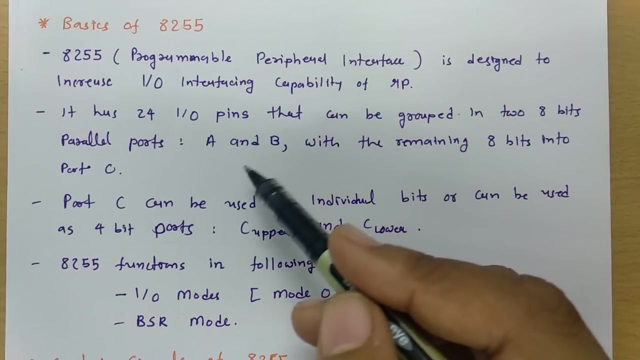 can be used as a group of four bits, with Upper group of C and lower group of C. Ultimately, in 8255, there are three ports: Ports A, port B and port C. port A and port B that can be used directly as parallel ports and port C that can be used as individual. 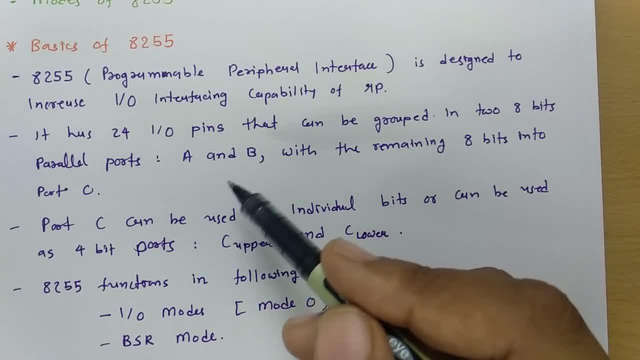 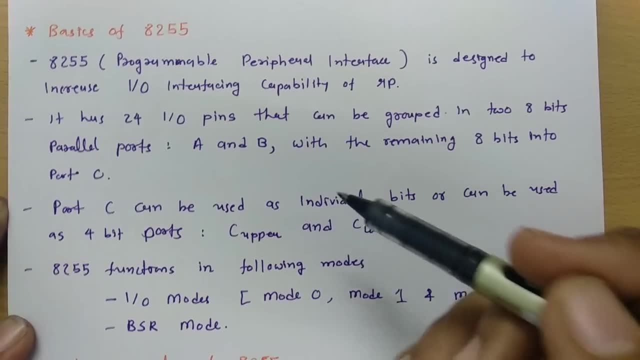 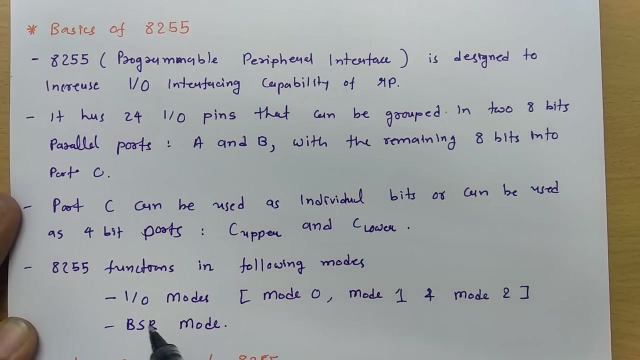 bits ¿And complete output interface per port C. And port C can be grouped further in upper C group and lower C group. 8255 functions in following modes: It functions in two different modes: input output mode and BSR mode. In input output mode there are another three modes like mode 0, mode 1 and mode 2.. 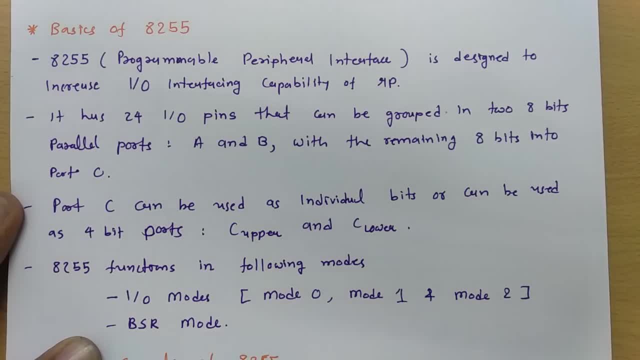 And in bits, BSR means bit set, reset mode. So these modes that I will be explaining in detail in this session, at the end of this session. So stay tuned. with this video You will be finding how these modes are functioning. 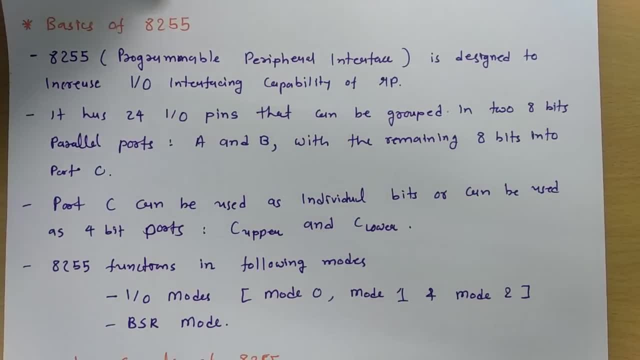 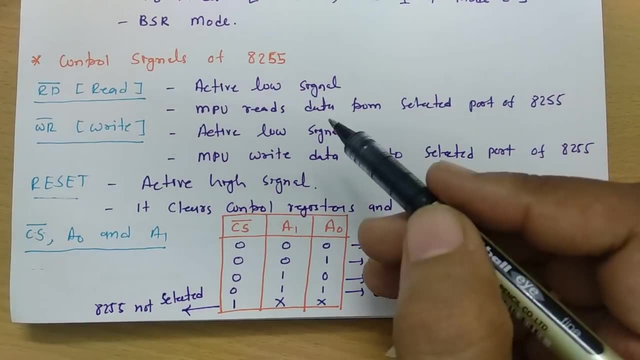 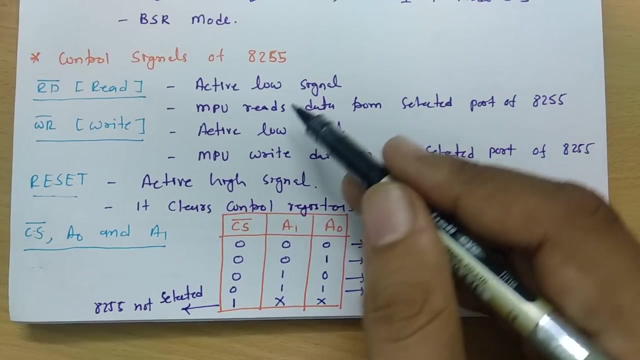 So it is little more interesting. Now see next part of this session, that is, control signals in 8255.. So when you see the IC of 8255, it has these control signals. So, which is so essential? Read bar signal. so that is active low signal. 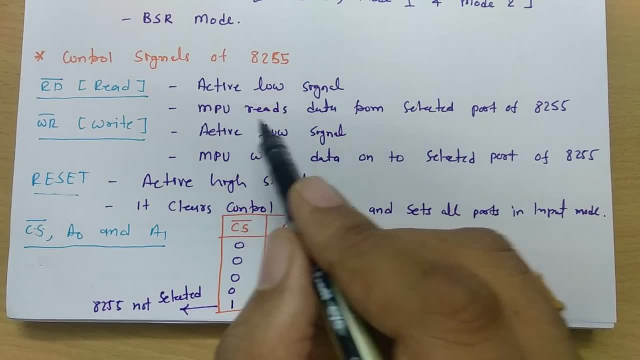 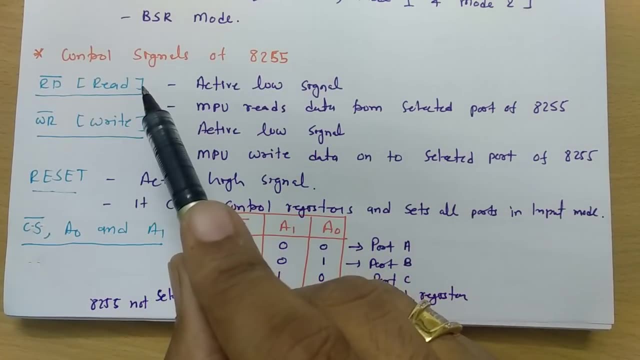 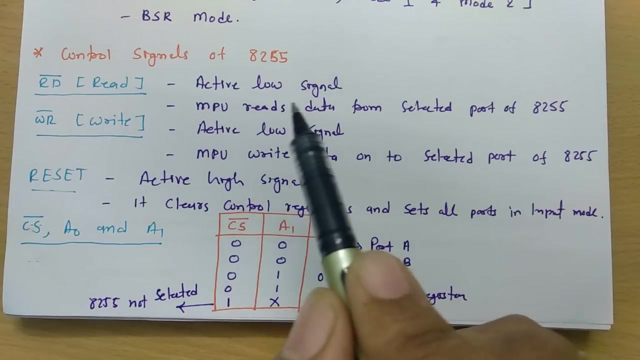 And that is been forwarded by microprocessor to read data from any of selected port. So when microprocessor sends read bar data means active low signal on this terminal. microprocessor wants to read data from the selected port. Write bar signal that is even active low signal. 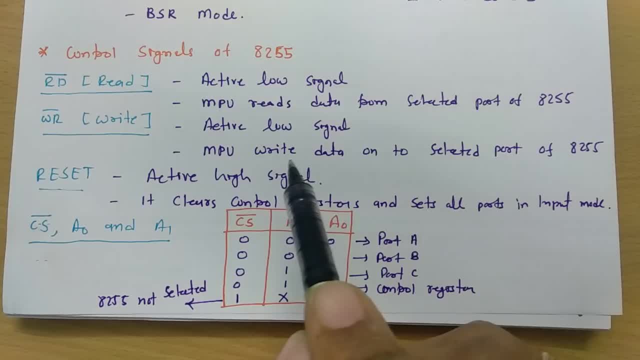 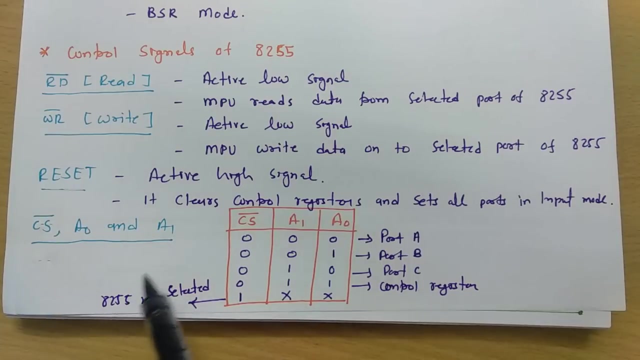 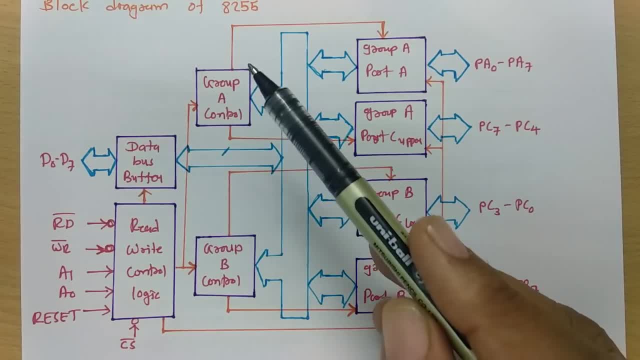 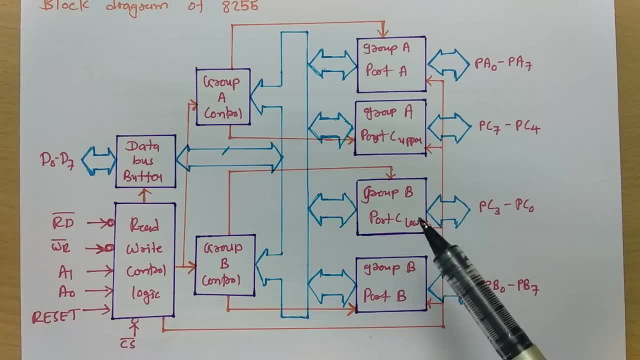 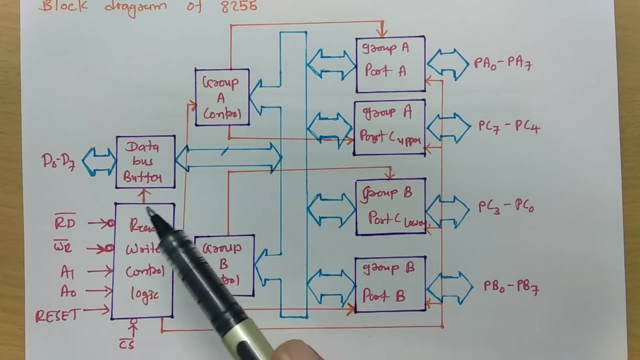 PC 7. so ultimately group A is having port A and upper port C and group B that is having control of port B and lower port C and this is what we are connecting it with: data transfer D0 to D7 and control signals: read bar, write bar A0, A1 and reset and chip select. so we have already discussed. 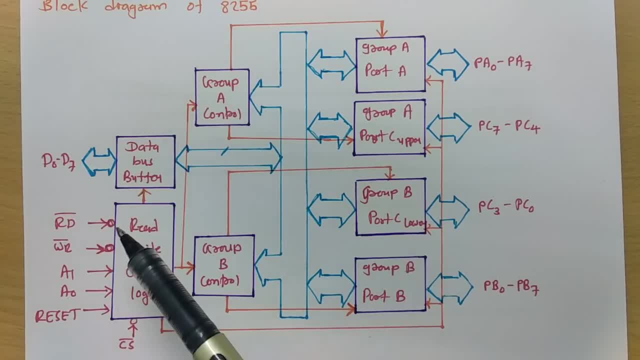 working of this terminals like read bar signal, that is to read data from selected port. write bar, that is to write data from selected port A0 and A1. that is, to select port A, port B and port C. if it is 0: 0, port A is getting selected 0: 1. port B is getting selected: 1: 0. port C is. 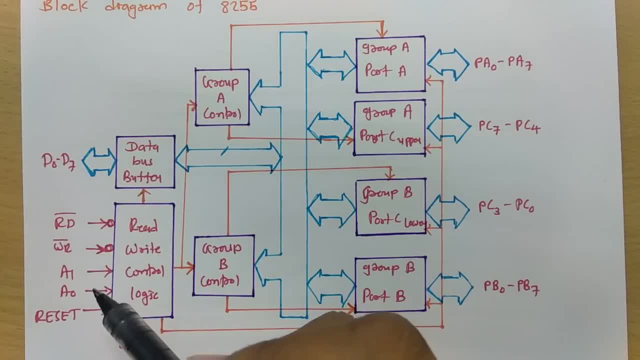 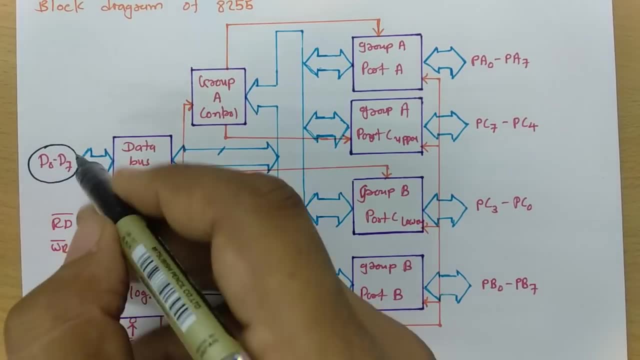 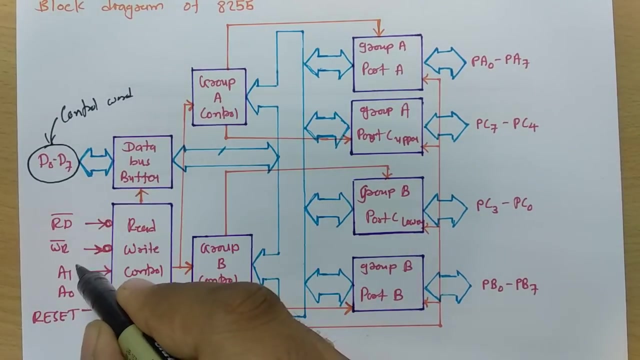 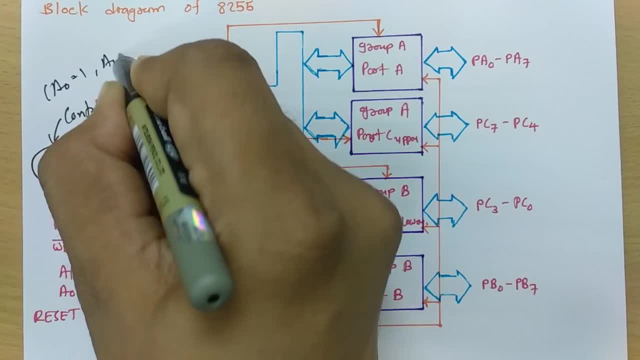 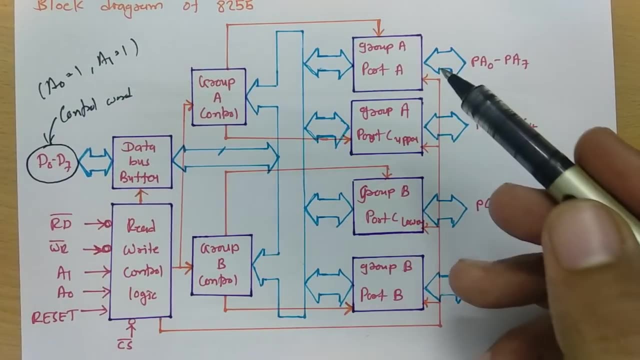 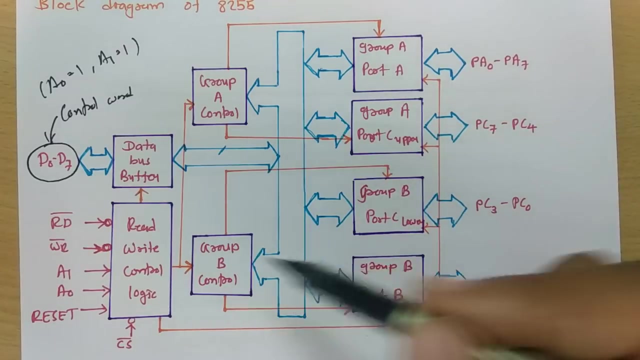 we will be having control word over here. so in control word we will be defining what type of mode of operation is happening right now with 8255 and based on that we can understand how this IC is functioning and in reset it is active high signal if it is been given to. 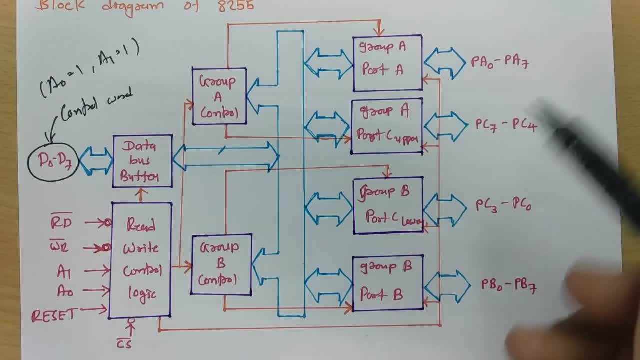 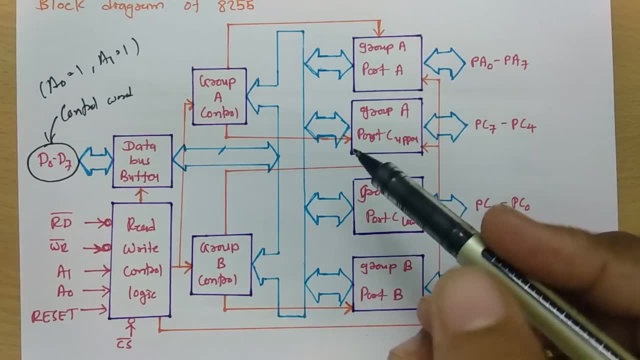 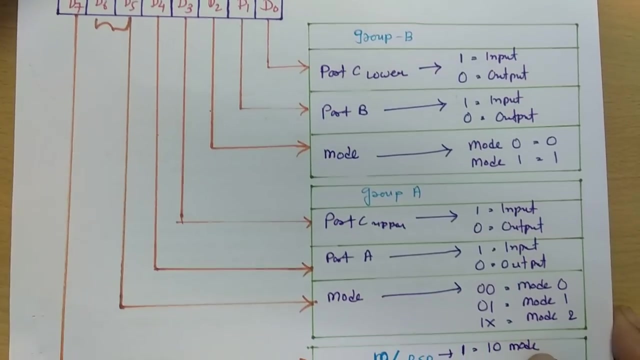 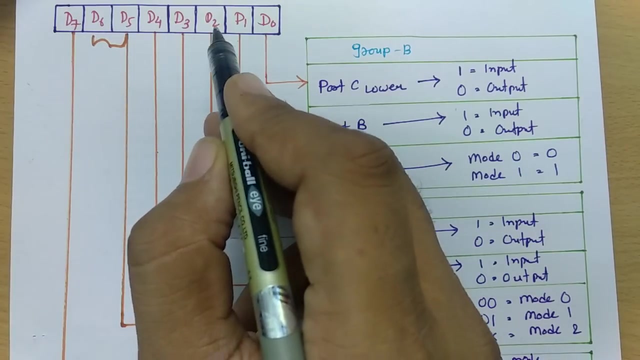 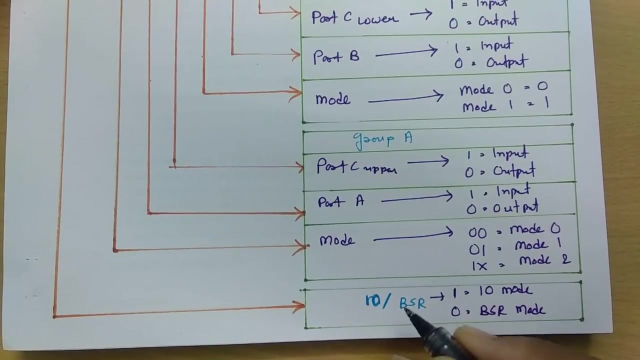 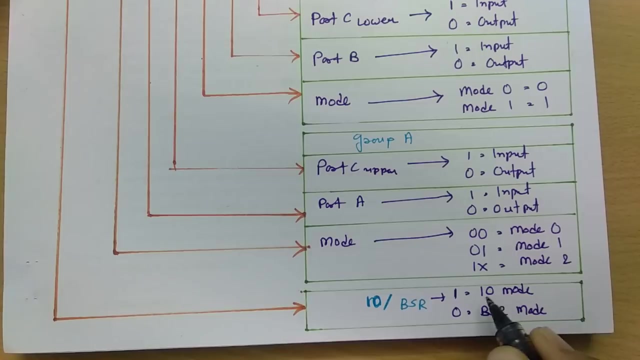 reset with 80, 50, all ports will function as input port, and so this is what the basic block diagram which is there with 8255. we are going to define a basic advice here: VDL, VDL, VDL, V, stol, one input output and BSR mode. If it is 1,, then 8255 will function in input output mode. 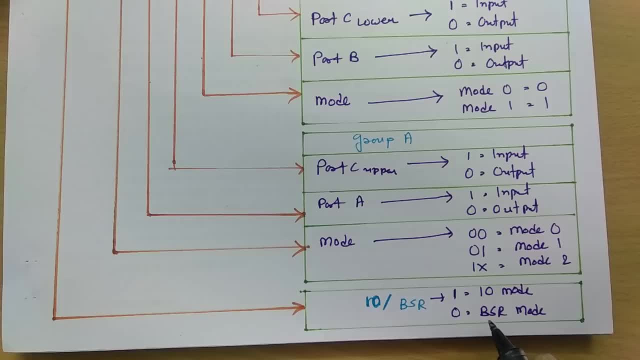 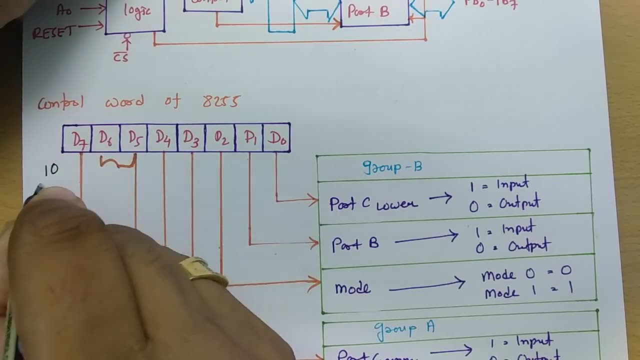 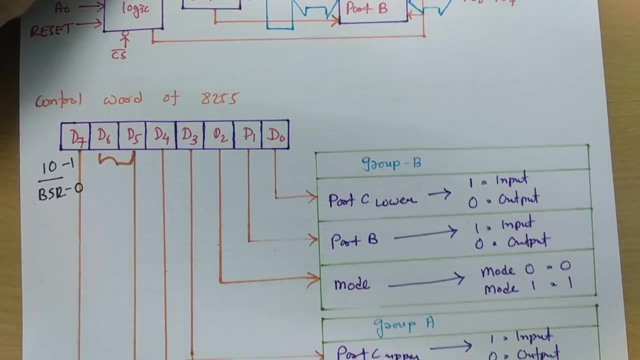 If it is 0,, then 8255 will function in BSR means bit set, reset mode. So this bit D7, that will define input output or BSR. If it is 1, then input output and if it is 0,, then BSR mode. that 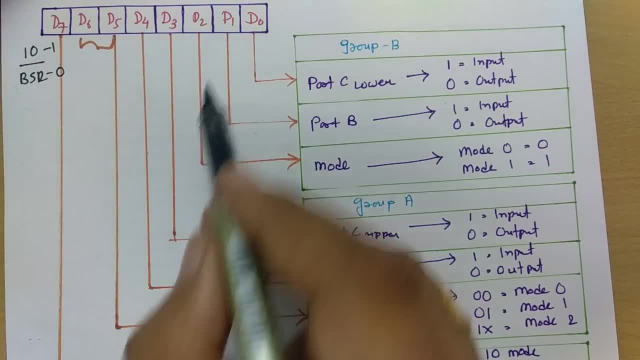 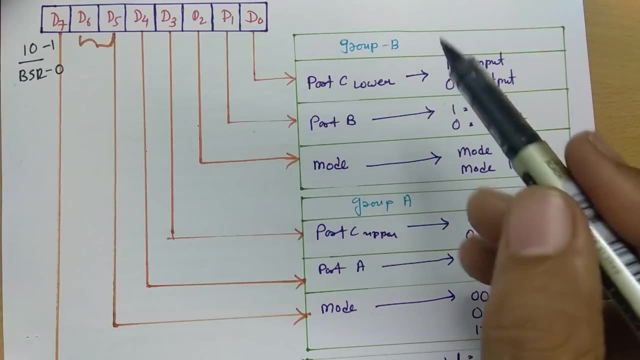 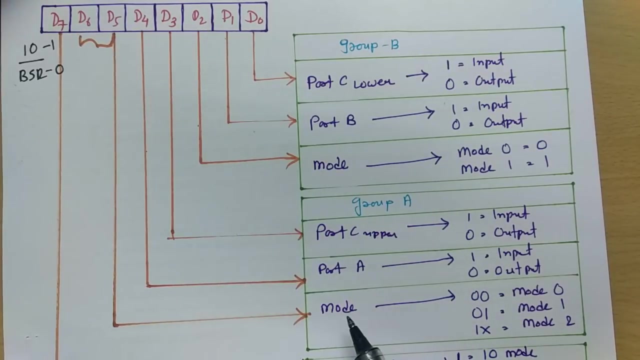 will get activated Now, as I have explained you, this IC can be bisected into two groups, group A and group B. Now see in group A this D5 and D6. that will define mode of operation. 00 will select mode 0,, 01 will select mode 1, and 1X means 1, don't care, that will select mode 2.. 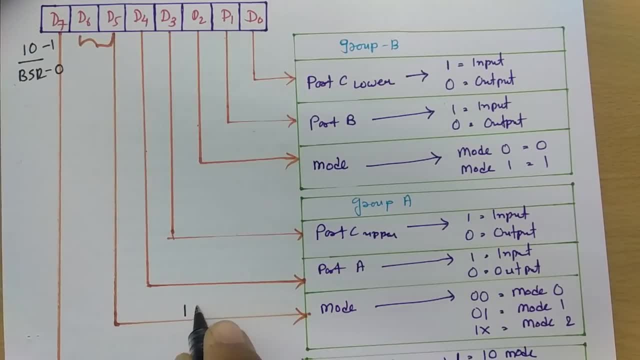 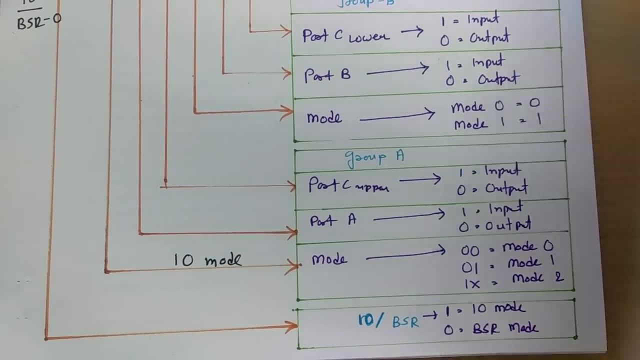 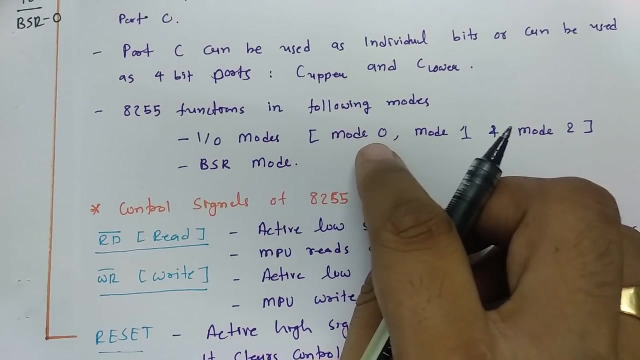 And this is what we are selecting it in input output mode. The reason is, I have already told like there are two types of modes: either input output mode, either BSR mode. So in input output modes there are three modes: mode 0,, mode 1 and mode 2.. And in BSR mode it is bit set reset mode. 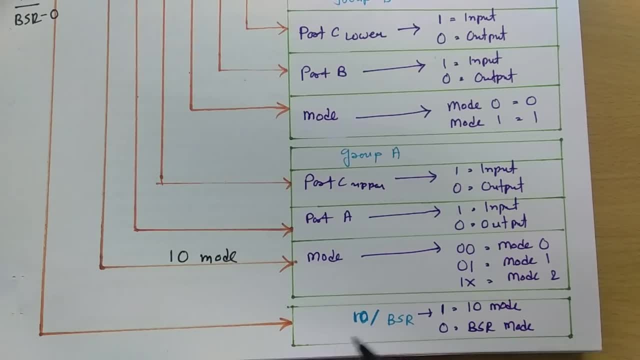 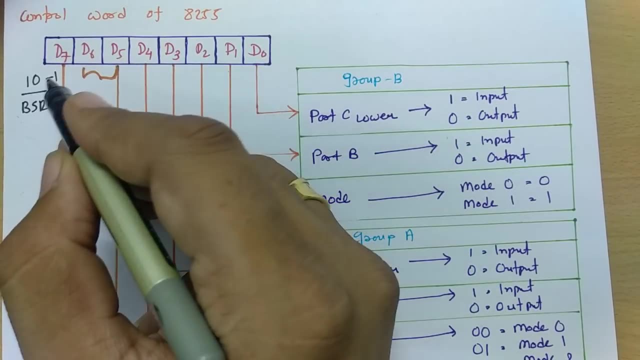 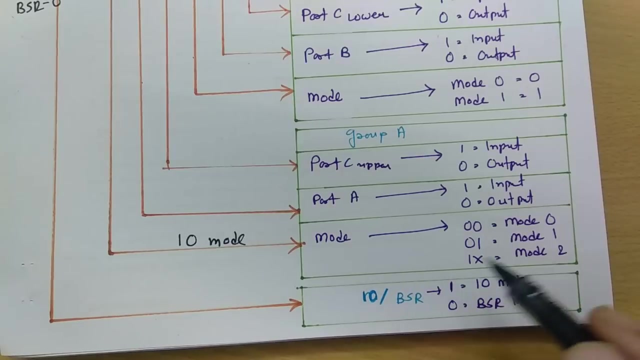 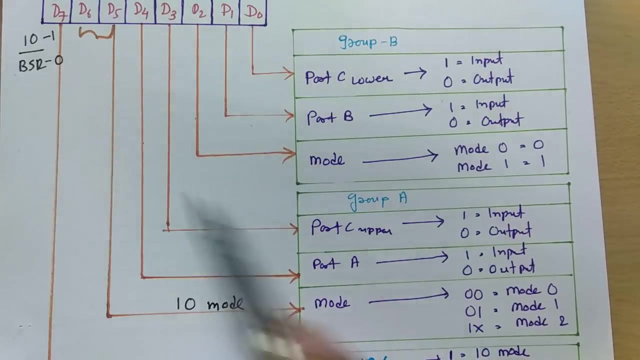 we will see that in detail. So if microprocessor- sorry microprocessor- is controlling 8255 with input output mode by placing D7 is equals to 1, then this group A, that can have mode 0, mode 1 and mode 2 by selecting D5 and D6. So if D5 and D6, that is 00. 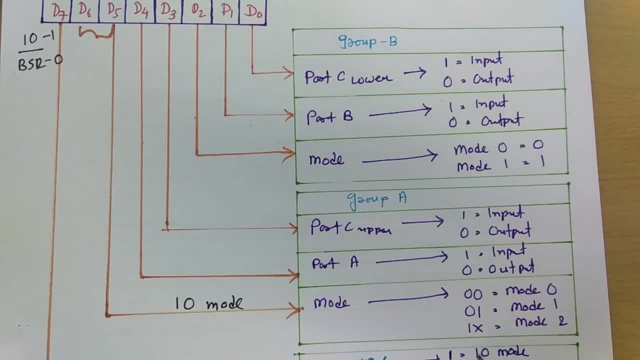 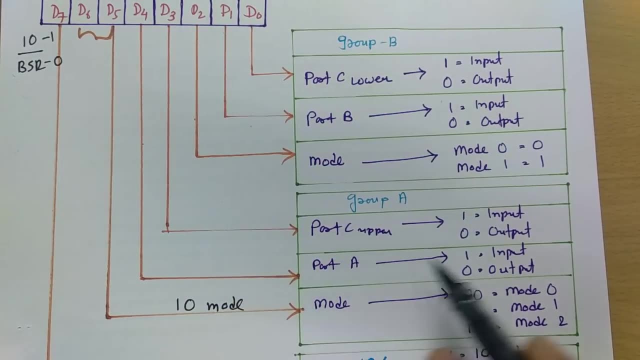 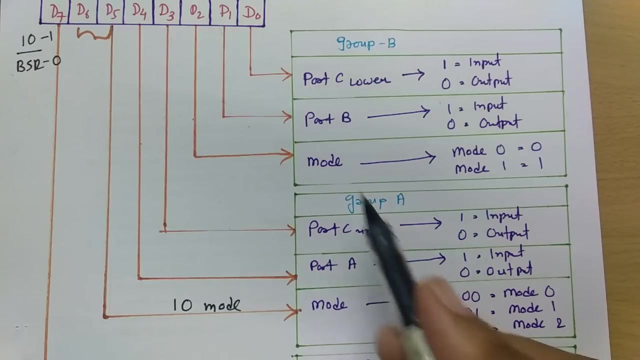 mode 0,, 01, mode 1, 1X, mode 2 will get selected And this D4 bit that is connected with port A. if it is 1,, port A will function as input. if it is 0,, port A will function as output And this D3 of group A. 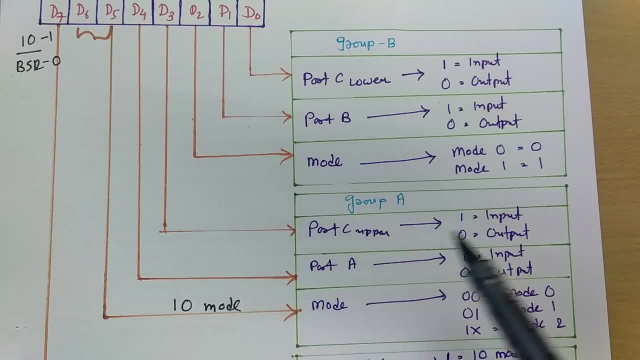 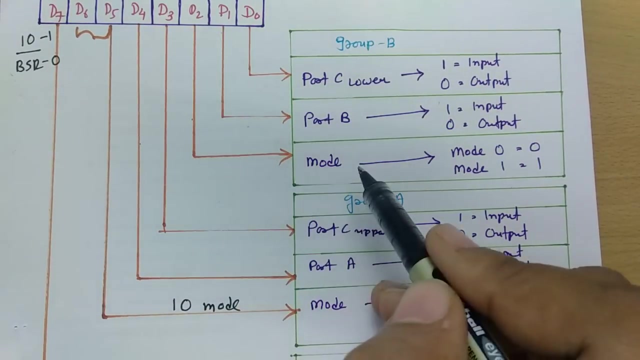 that is connected with upper port of C, which will be having: 1 is equals to input, upper port, 0 is equals to output of C. upper port For group B: control this D2 bit that will select mode. if it is 0, then mode 0 will get selected. If it is 1,, then mode 1 will get selected. 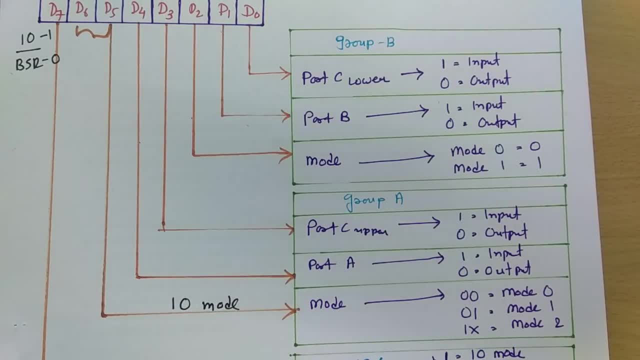 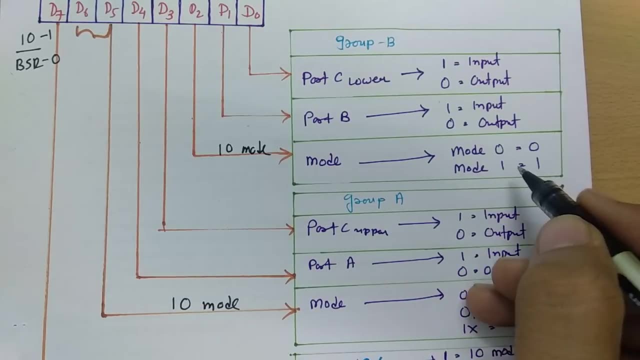 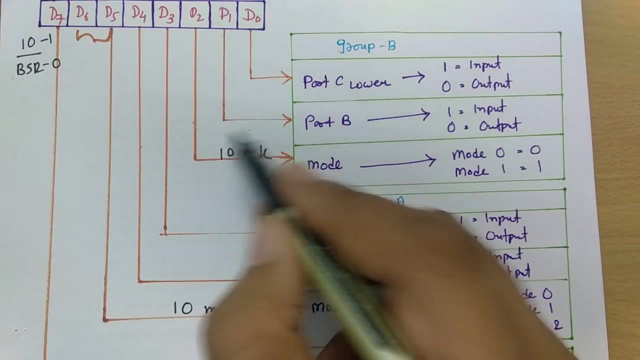 So in group B we cannot have mode 2.. In group E, input output mode, there are only two modes: mode 0 and mode 1.. 0 will result into mode 0 and 1 will result into mode 1.. This D1 bit. 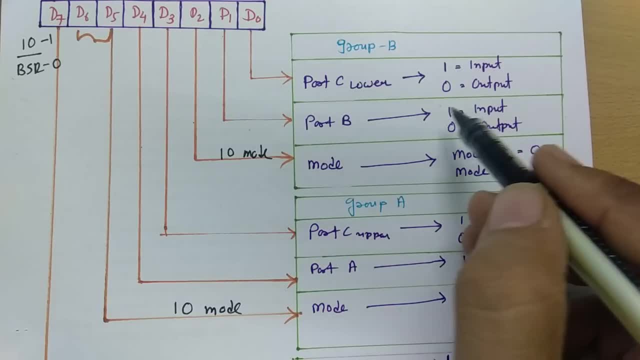 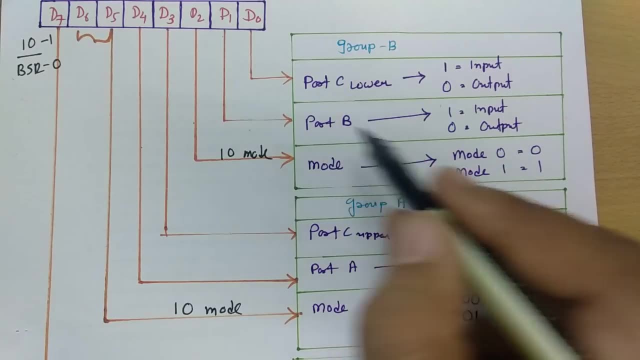 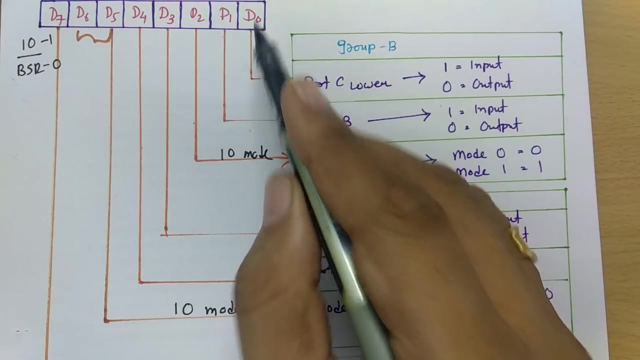 that is, selecting port B as input as if it is 1.. If it is 0, then it will get selected with output port. So port B will be output in case of 0 and 1 will result into input port And this D0 that will make. 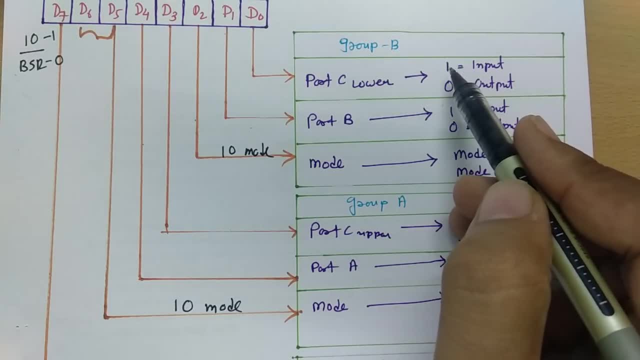 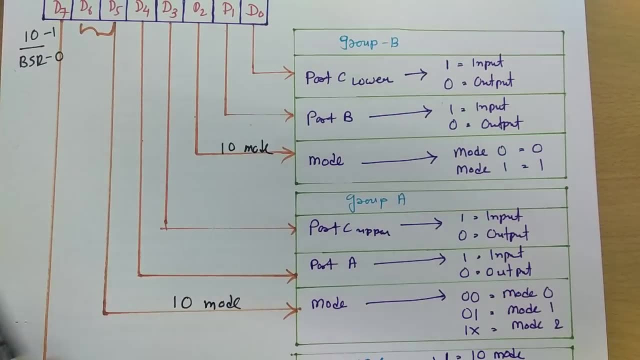 C, lower port, as input port. if it is 1 and if it is 0, then it will be output port. So this is what about control, word of 8255.. Now let us try to understand what is this control at 8255. 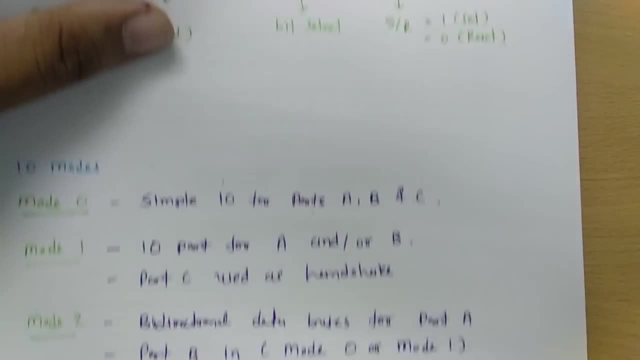 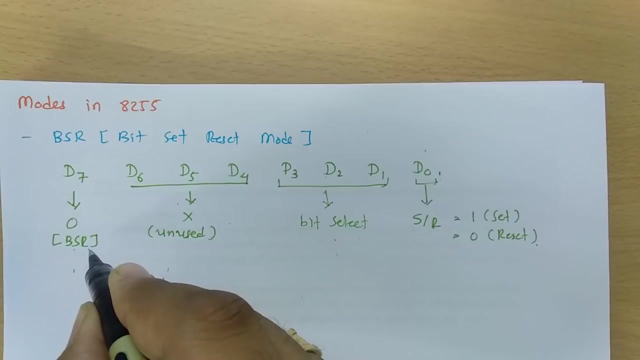 Now let us try to understand what is this control impossible? So this is: what about control, word of 8255.. Now let us try to understand what is this control impossible, understand how many modes are there. so see, as I have told this D7 bit, that will make. 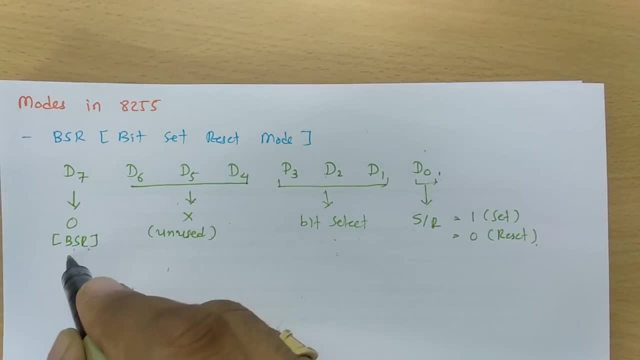 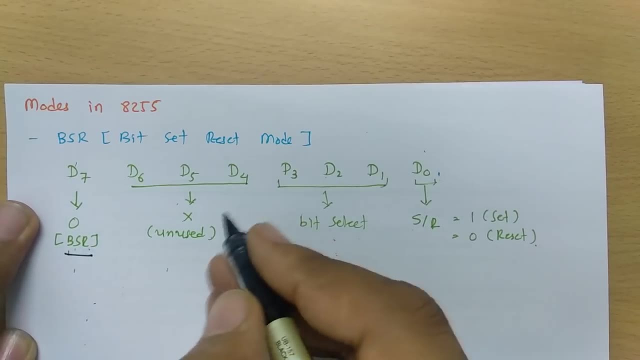 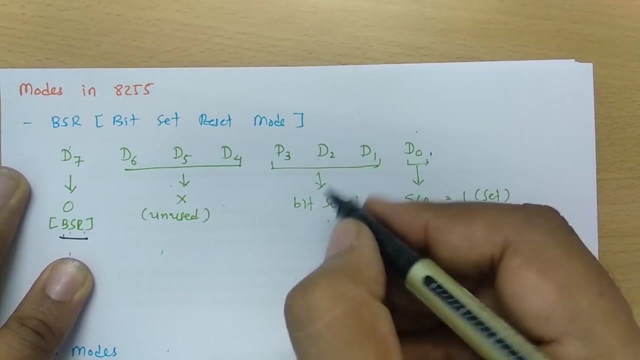 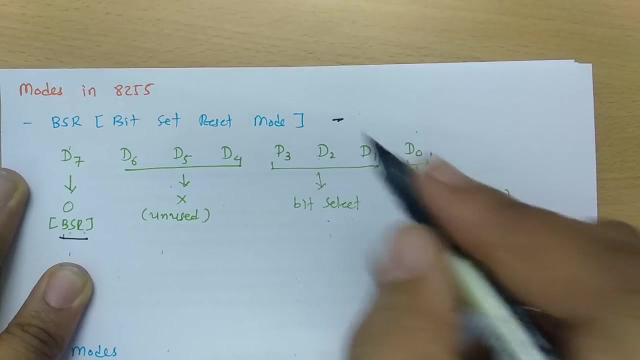 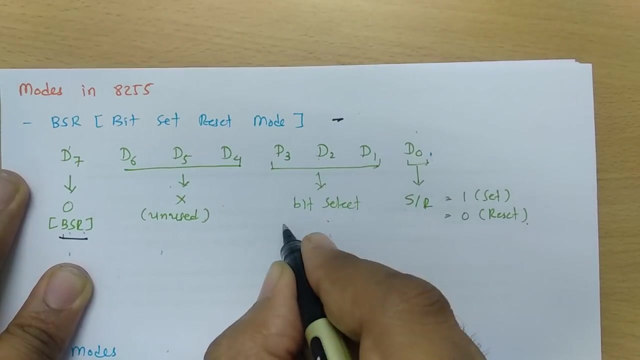 BSR mode. so if it is 0, then we can say 8255. that is there in BSR mode now where in BSR means beat set reset mode. so what we will be doing is we will be setting port C as beat set reset mode. now see how this D1, D2, D3, that will select bit. so if it is 0, 0, 0, it will. 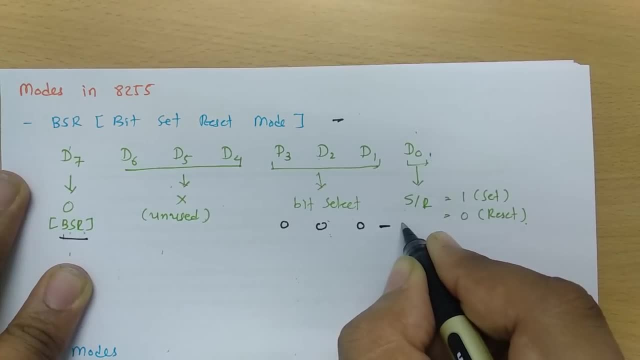 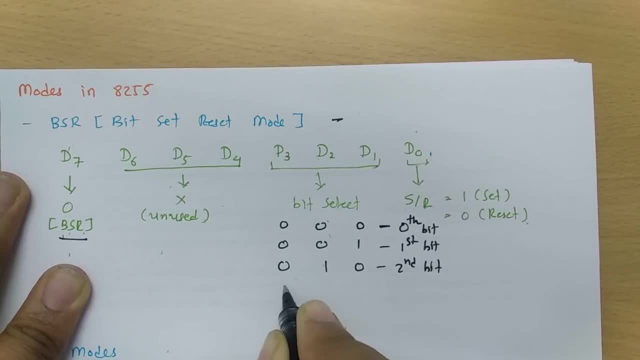 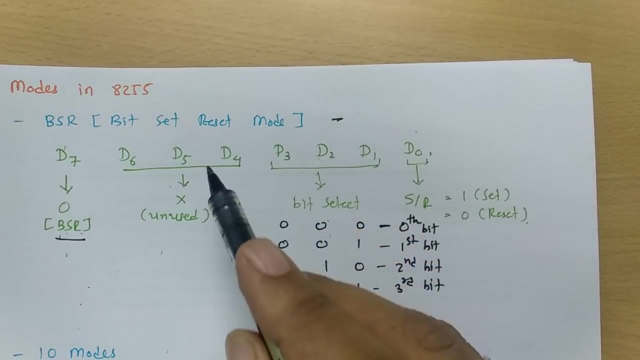 selecting second bit. if it is 0 1- 1, it will be selecting third bit. likewise, if it is 1 1- 1, it will be selecting seventh bit of port C. so any bit of port C that will get selected by using d1, d2 and d3, this d4, d5 and d6 that is unused. now to